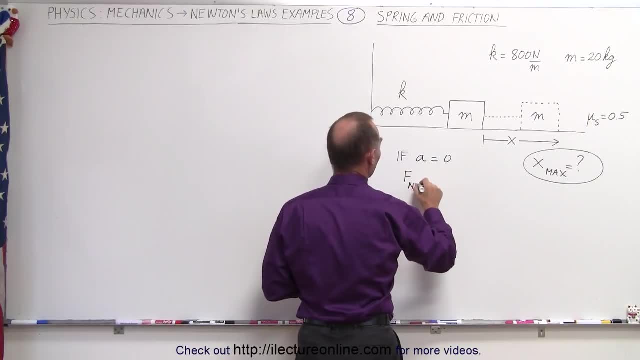 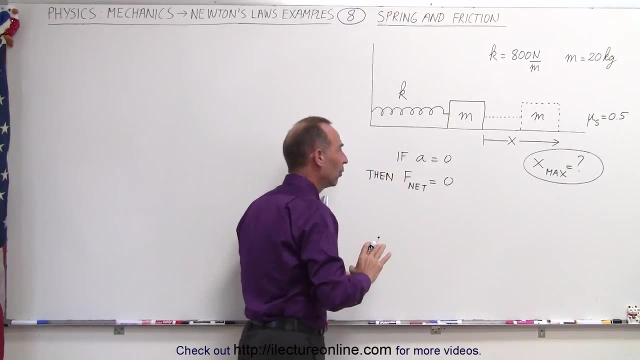 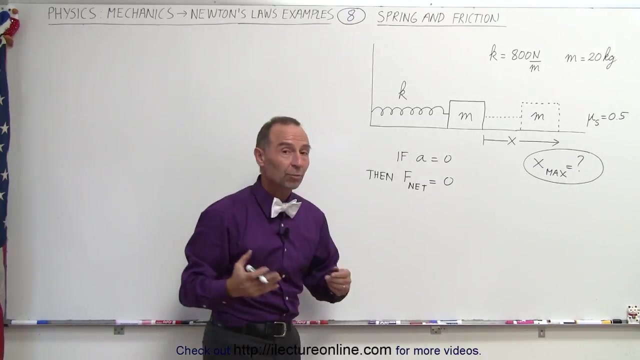 is equal to 0, then we know that the net force must also equal to 0. So if that, then this: In other words, we're going to identify all the forces acting on the mass when it's extended out to this distance and then see what the conditions must be so that the object will now not start. 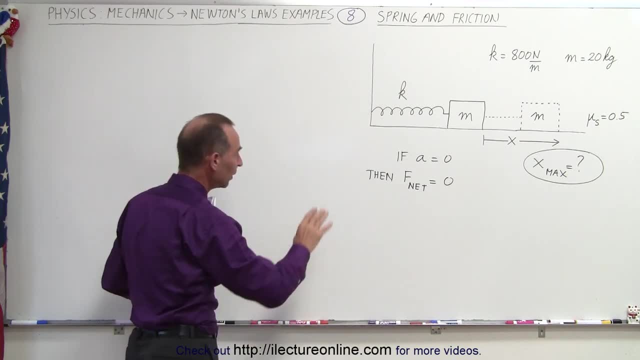 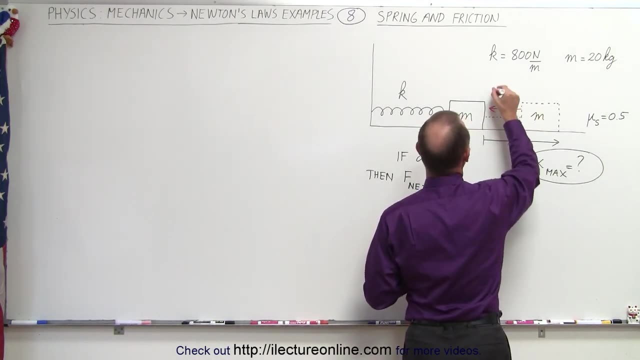 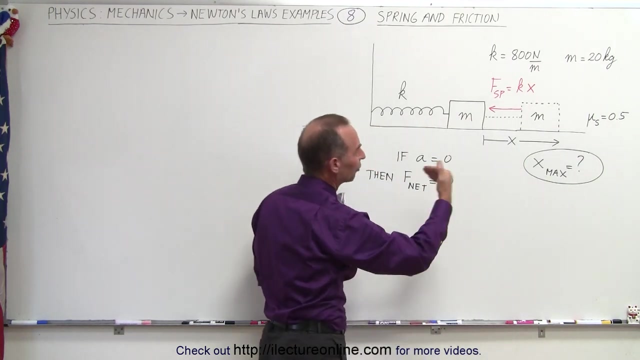 accelerating back towards its equilibrium point. So once it's over there, we then can say that well, the spring is going to be So. that's force holding to the right, so force of the spring, and that will be equal to the magnitude of the K, the coefficient of the spring times the distance that it's been extended. 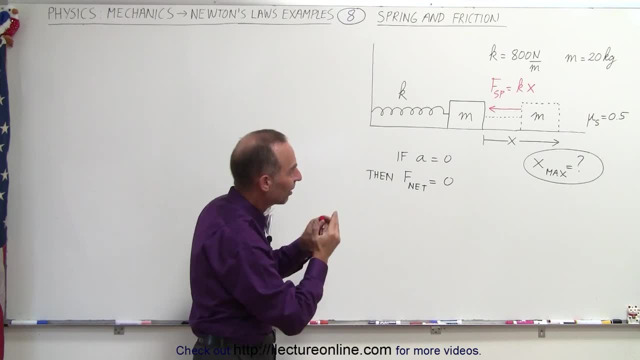 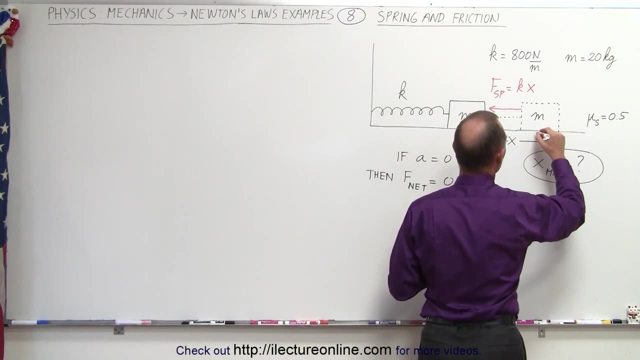 And notice that the force is acting to the left and the magnitude of the force is the spring, constant times, the distance away from the equilibrium point And at the same time, we also know that there is a force due to gravity, which is Mg. 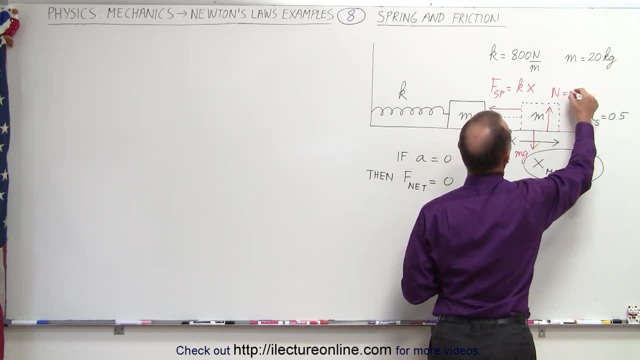 which means there's a normal force acting here on the left midpoint. here The force orders the situation, force pushing back n, which is going to be equal to mg. and then what will prevent the mass from accelerating to the left? well, it would be a friction force to the right, force friction. 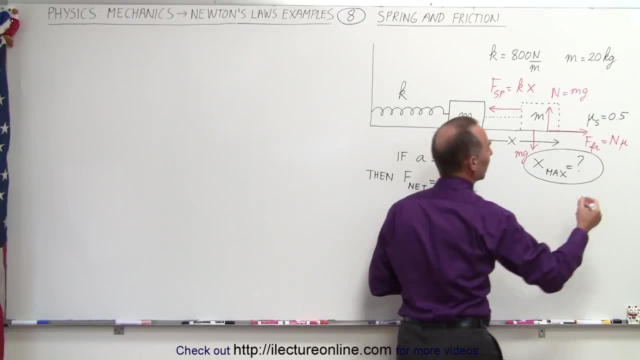 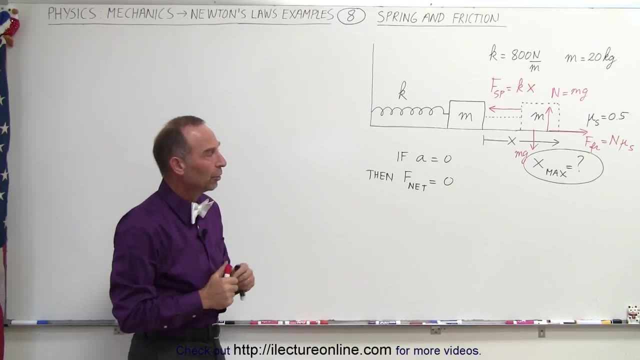 which is going to be equal to the normal force times, mu, and in this case it'll be the static coefficient of friction, if we pull the mass outward and then hold it stationary before we let go, so that that way we deal with the static coefficient of friction, and so we can say then: is 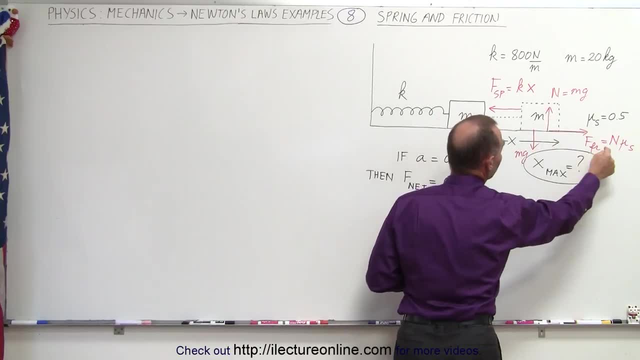 that nothing will move. so the block will stay in place as long as the maximum value of the coefficient of the friction force is greater or equal to the force caused by the spring. so we know that there will be a net force equal to zero if this force is less than the maximum. 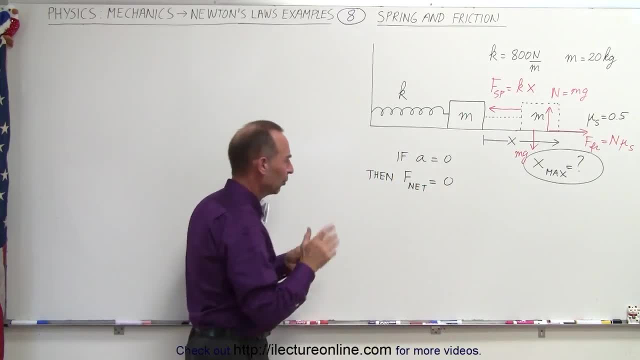 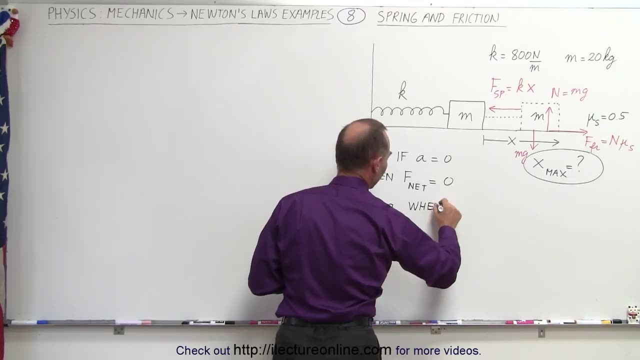 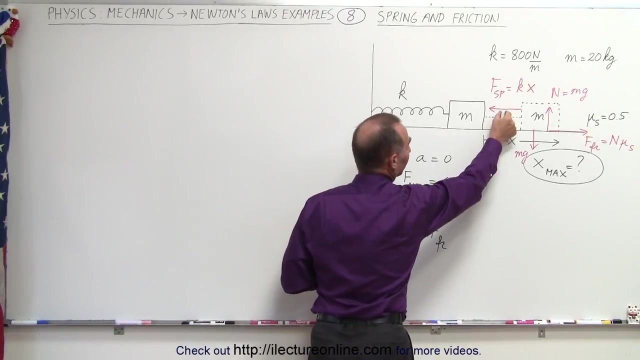 force the friction could be. so let's understand that a little bit more. so what i said was that no acceleration so no a when, when, when the force of the spring is less than or equal to the force caused by the friction- because what happens is, let's say that you pull it out just a little bit- then the force of the 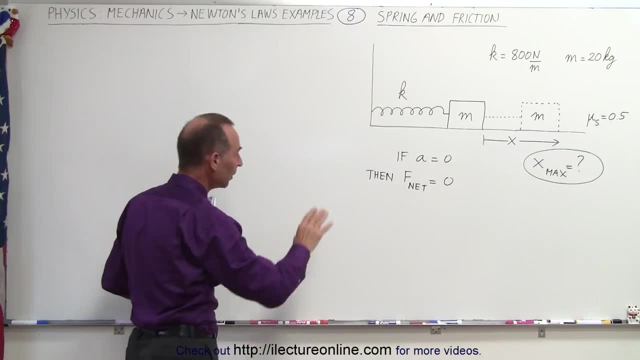 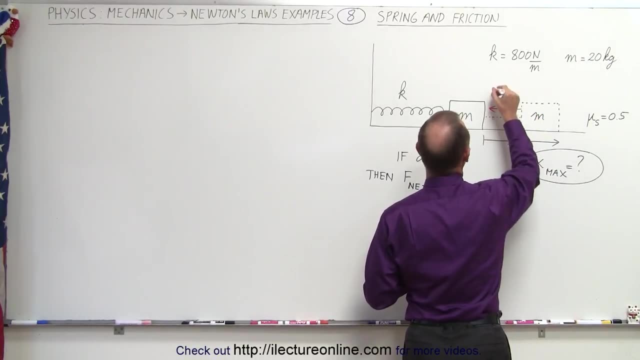 accelerating back towards its equilibrium point. So once it's over there, we then can say that well, the spring is going to be pulling to the right. so that's force of the spring, and that will be equal to the magnitude of 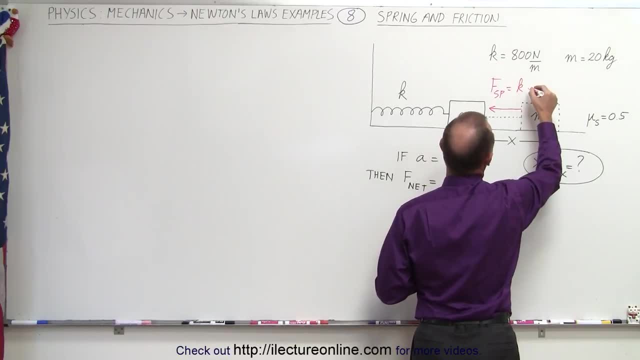 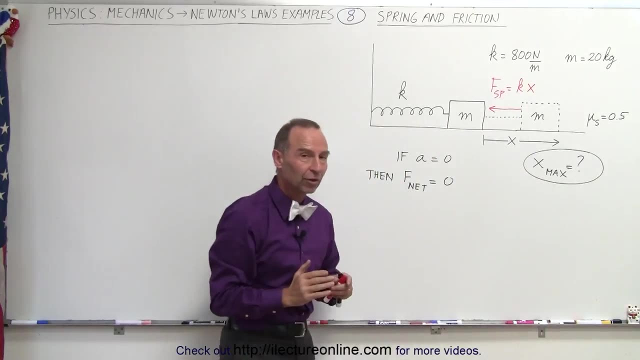 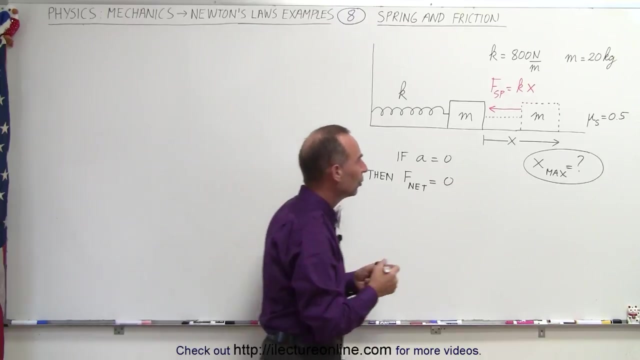 the k, the coefficient of the spring times, the distance that it has been extended, And notice that the force is acting to the left and the magnitude of the force is the spring constant times, the distance away from the equilibrium point. And at the same time we also 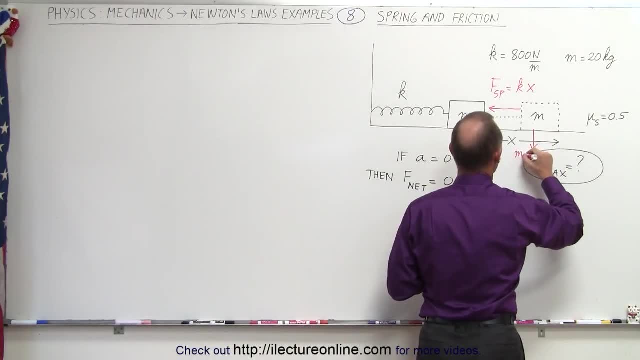 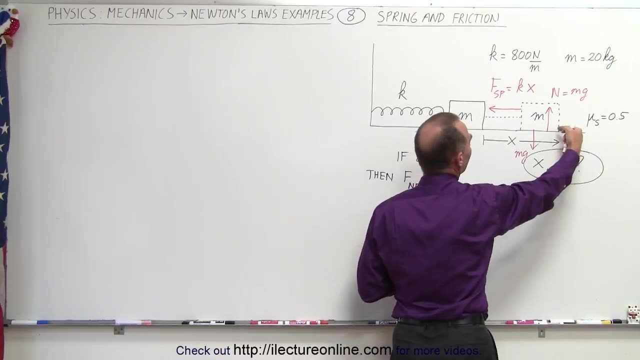 know that there is a force due to gravity which is mg, which means there is a normal force in the force pushing back n, which is going to be equal to mg. and then what will prevent the mass from accelerating to the left? well, it would be a friction force to the right, force friction. 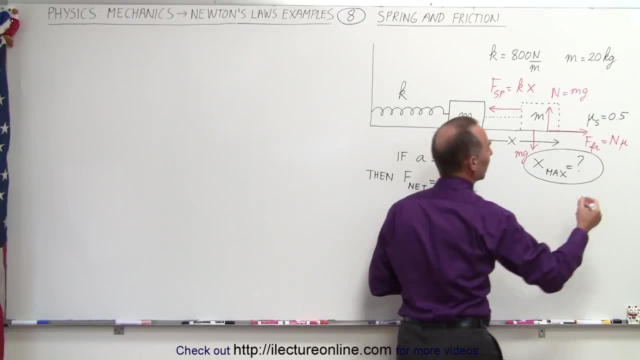 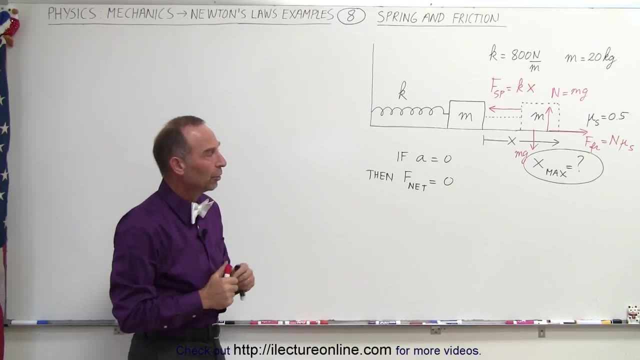 which is going to be equal to the normal force times, mu, and in this case it'll be the static coefficient of friction, if we pull the mass outward and then hold it stationary before we let go, so that that way we deal with the static coefficient of friction, and so we can say then: is 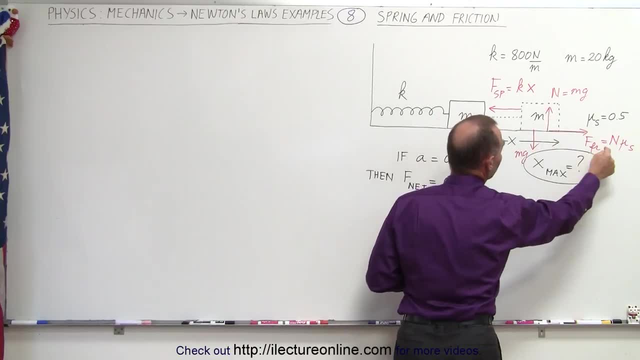 that nothing will move. so the block will stay in place as long as the maximum value of the coefficient of the friction force is greater or equal to the force caused by the spring. so we know that there will be a net force equal to zero if this force is less than the maximum. 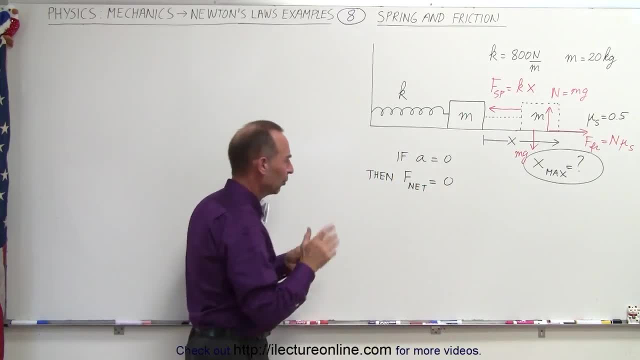 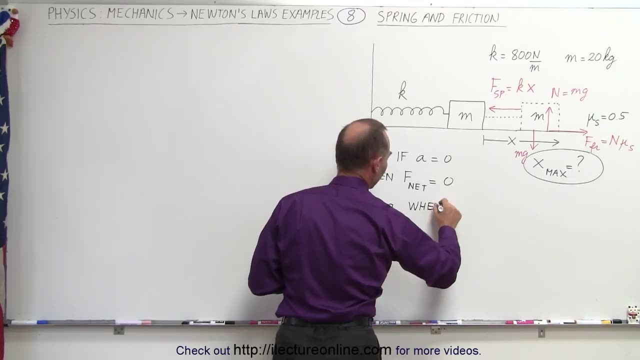 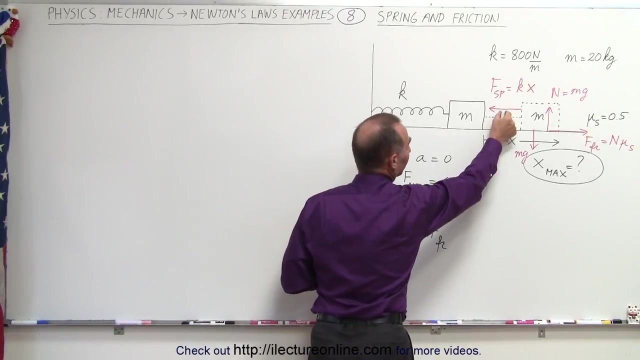 force the friction could be. so let's understand that a little bit more. so what i said was that no acceleration so no a when, when, when the force of the spring is less than or equal to the force caused by the friction- because what happens is, let's say that you pull it out just a little bit- then the force of the 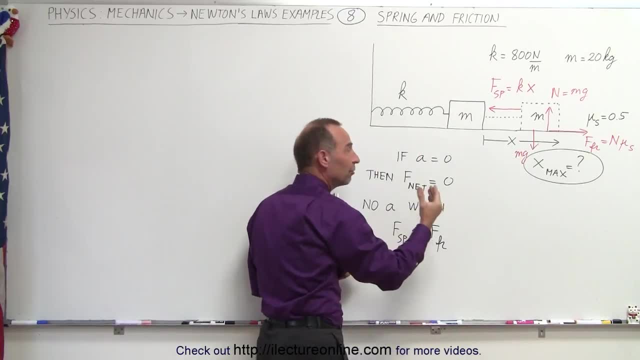 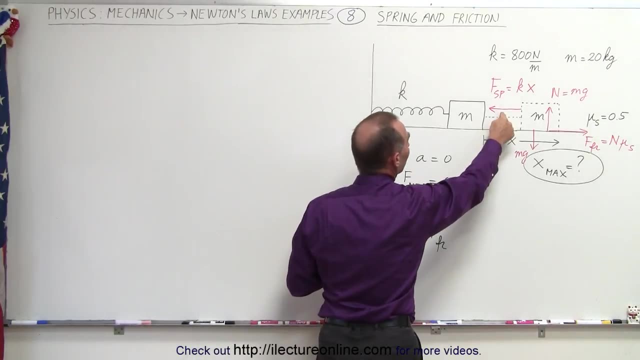 spring will be very small, and then the coefficient of, then the friction force will be small as well. in other words, the friction force can only be equal to or smaller than the force that you apply, because as you continue to, as you continue to pull the mass out of the spring, the force will be. 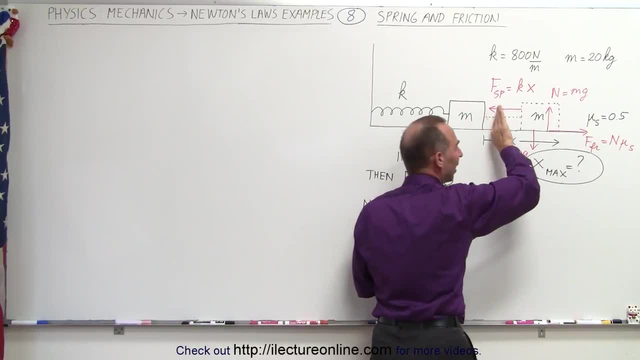 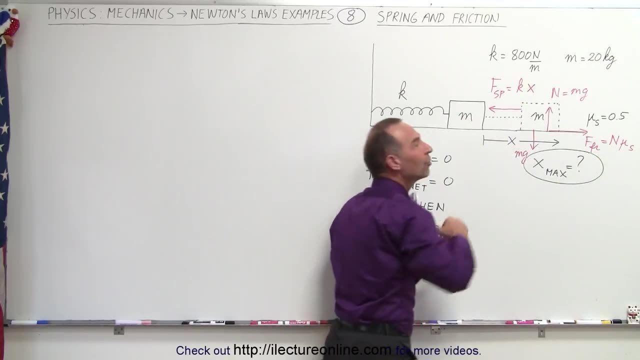 stronger. so then you'll see that the resistance will continue to to pull the block further outward. i'm pointing the wrong direction. as you continue pulling the block further outward, you will increase this value, and that means that this will simply respond to that force. so the friction force. 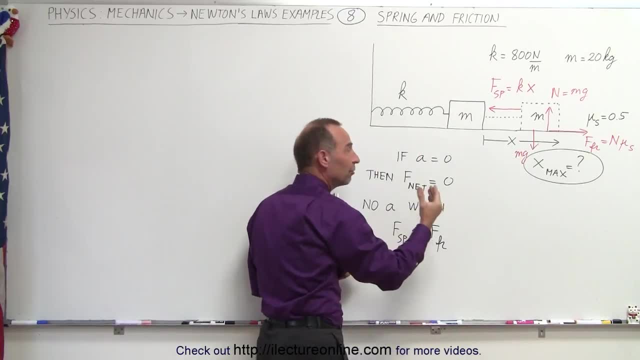 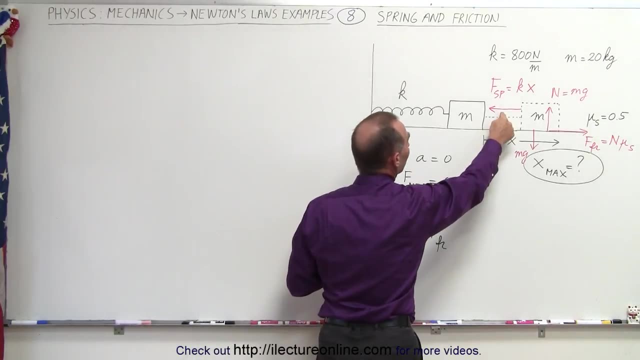 spring will be very small, and then the coefficient of, then the friction force will be small as well. in other words, the friction force can only be equal to or smaller than the force that you apply, because as you continue to, as you continue to pull the mass out of the spring, the force will be. 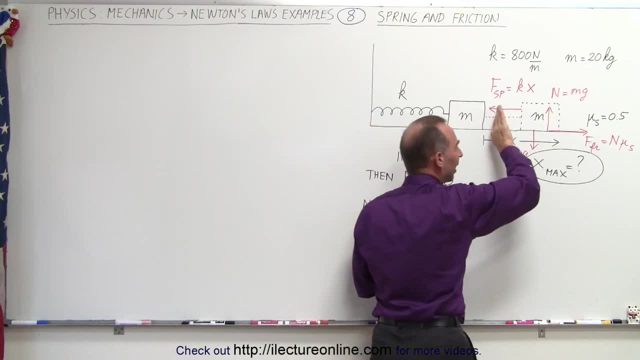 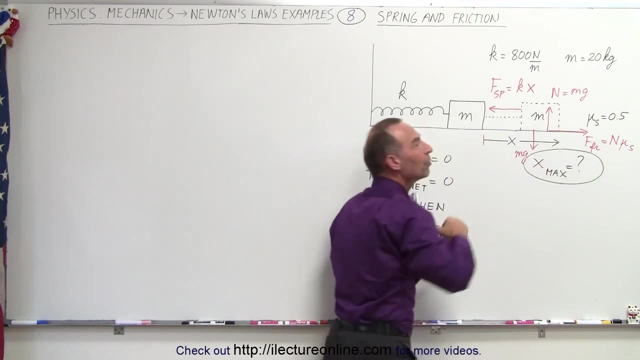 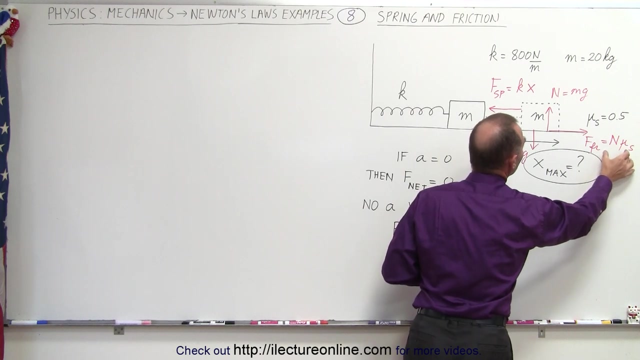 greater. continue to pull the block further, where I pointed the wrong direction. as you continue pulling the block further outward, you will increase this value and that means that this will simply respond to that force. so the friction force is actually a reactionary force loaded which the value of the friction force will always be equal to the value of the force it. 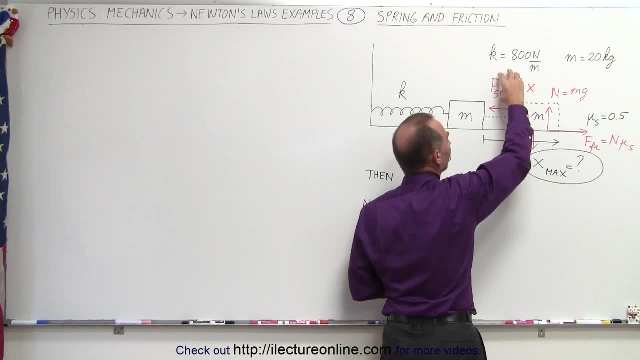 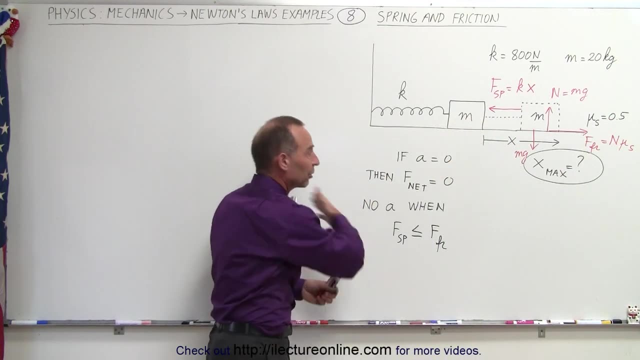 is spring until you pull it out so far that the value of the force of the spring becomes larger than the maximum that the friction force can be, and at that point point the object will accelerate to the left. so, in other words, the friction force as you increase. 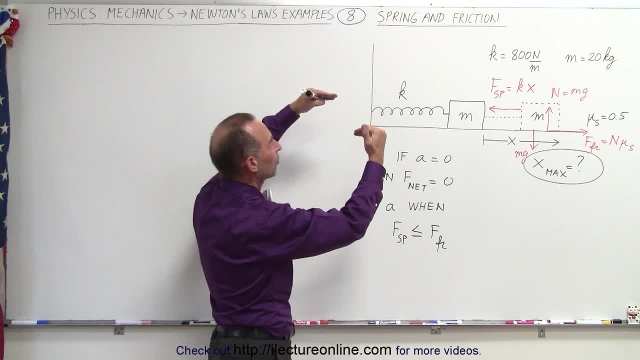 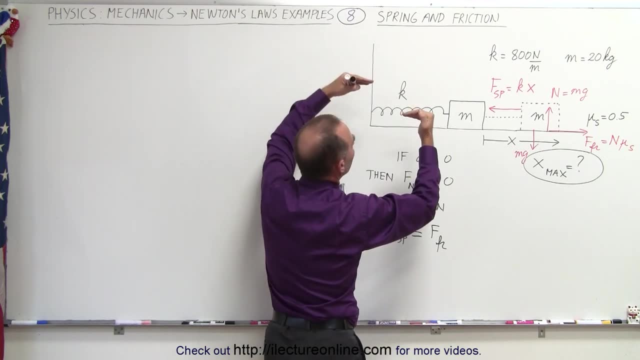 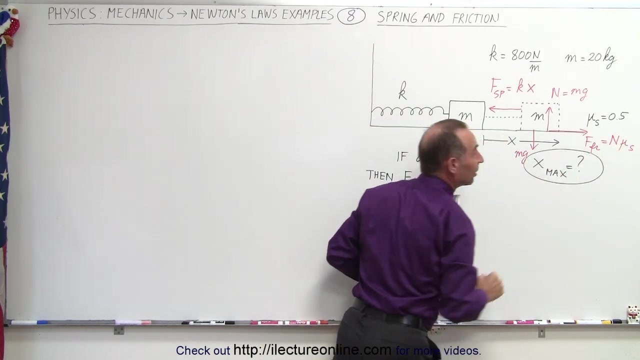 the force on the spring, the friction force will increase. increase the force in the spring, the friction force will increase, become equal as you pull the block further and further out, but eventually the force of spring becomes so high that the friction force cannot match it anymore, because the maximum friction force can be is equal to this. that's the key of the friction force, the 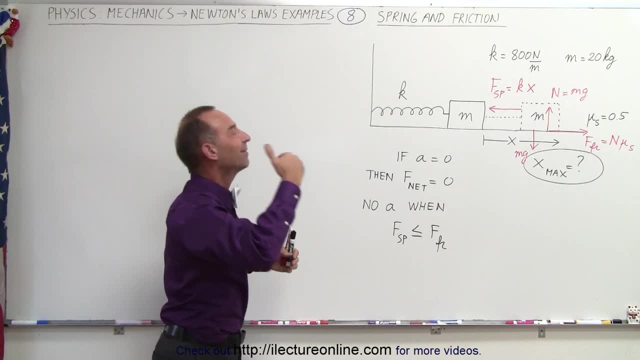 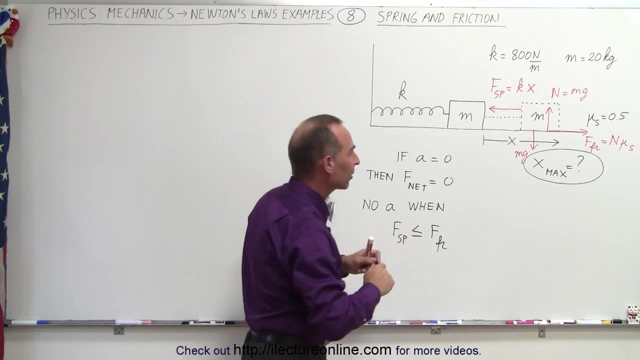 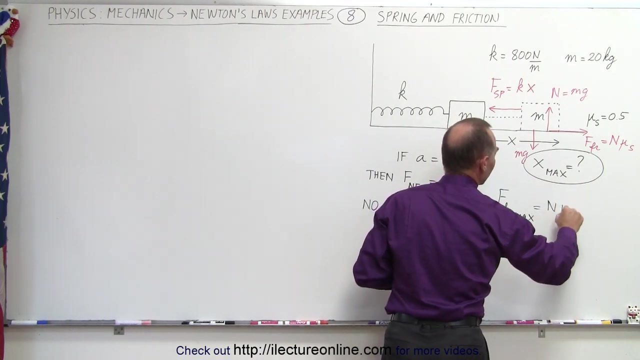 friction force is the reactionary force but can never exceed this particular value. it can never exceed n times mu sub s. so let's find the maximum friction force. so the friction force maximum is equal to the normal force times mu, which is equal to mg times mu, and of course that would be. 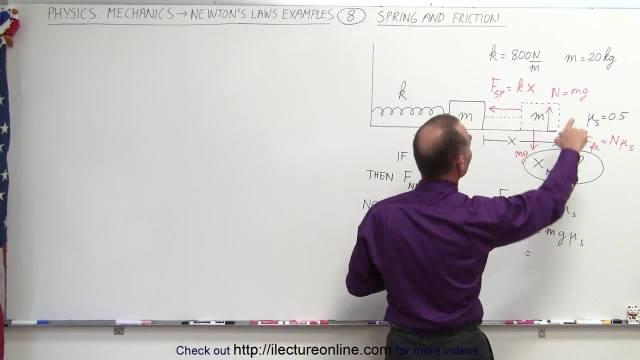 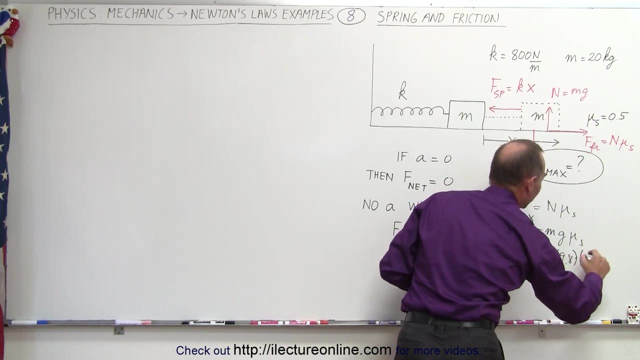 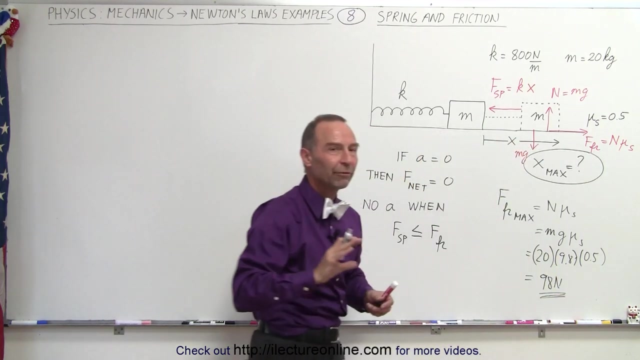 the static coefficient of friction. so this case would be: the mass is 20 kilograms. so 20 kilograms times 9.8 meters per second, square times mu sub s, which is 0.5, so this is equal to 98 newtons. so that's the maximum the friction force can be. now let's find out what x will be when the friction 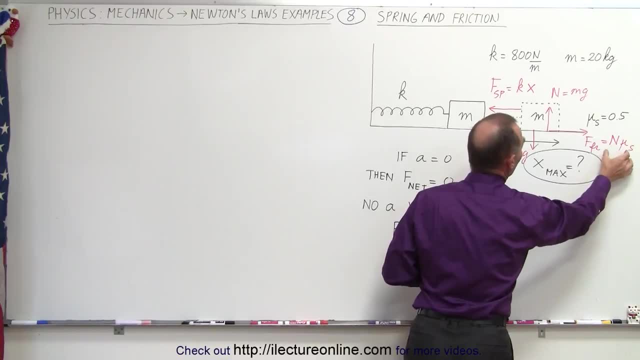 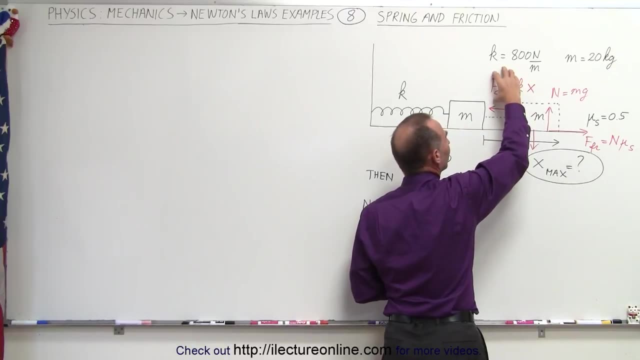 is actually a reactionary force, but other words, the value of the friction force will always be equal to the value of the force of the spring until you pull it out so far that the value of the force of the spring becomes larger than the maximum that the friction force can be, and at that. 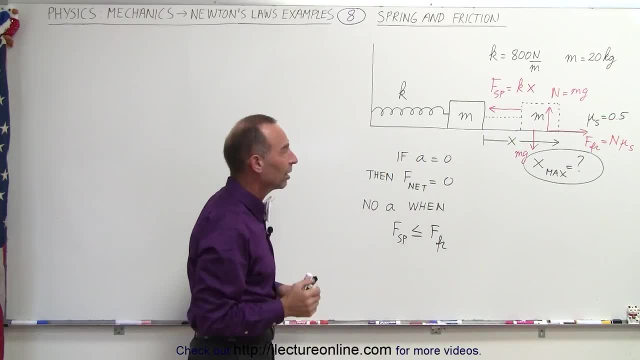 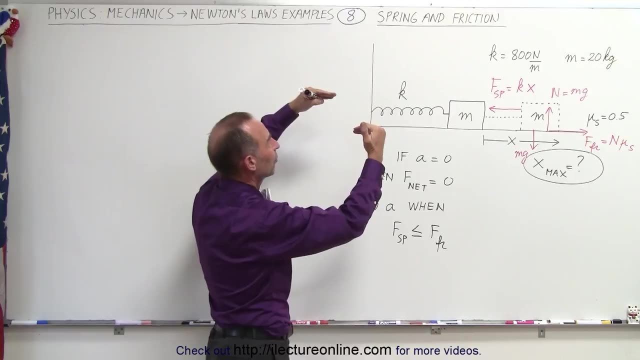 pointris, that moment he pulls out more force so that this power is the reactionary force, the exhaust point, the object will accelerate to the left. so in other words, the friction force: as you increase the force on the spring, the friction force will increase. increase the force in the spring, the 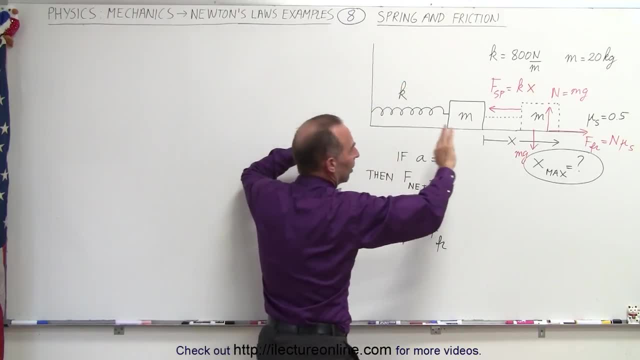 friction force will increase, become equal as you pull the block further and further out, but eventually the force of spring becomes so high that the friction force cannot match it anymore, because the maximum friction force can be is equal to this. that's the key of the friction force, the 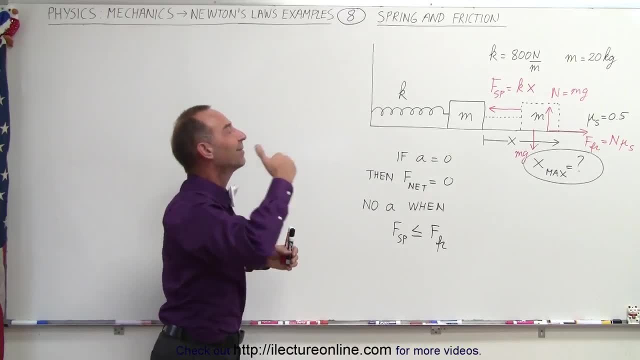 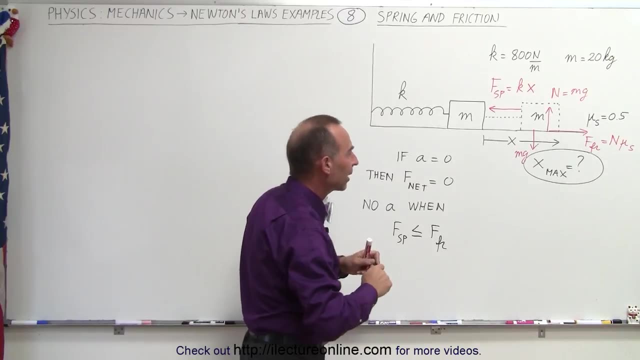 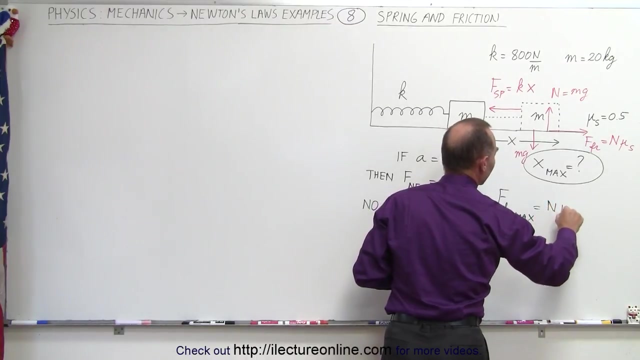 friction force is the reactionary force but can never exceed this particular value. it can never exceed n times mu sub s. so let's find the maximum friction force. so the friction force maximum is equal to the normal force times mu, which is equal to mg times mu, and of course that would be. 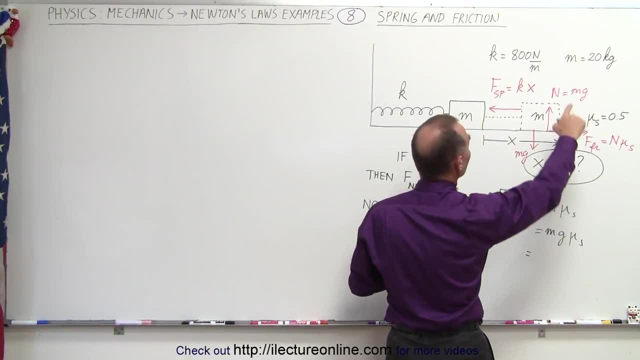 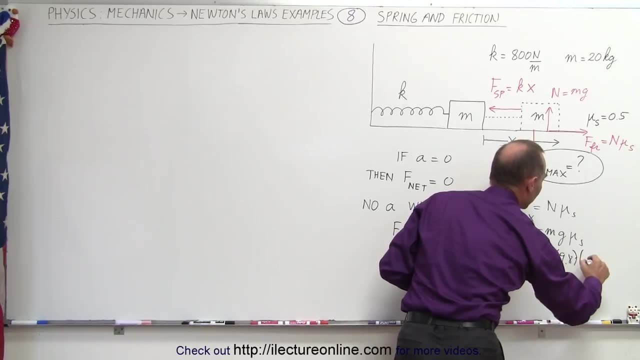 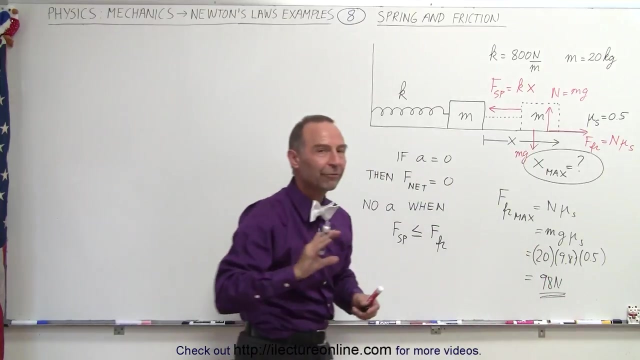 the static coefficient of friction. so this case would be: the mass is 20 kilograms. so 20 kilograms times 9.8 meters per second, square times mu sub s, which is 0.5, so this is equal to 98 newtons. so that's the maximum the friction force can be. now let's find out what x will be when the friction 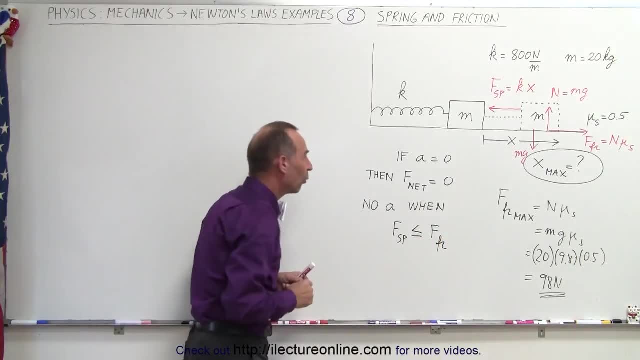 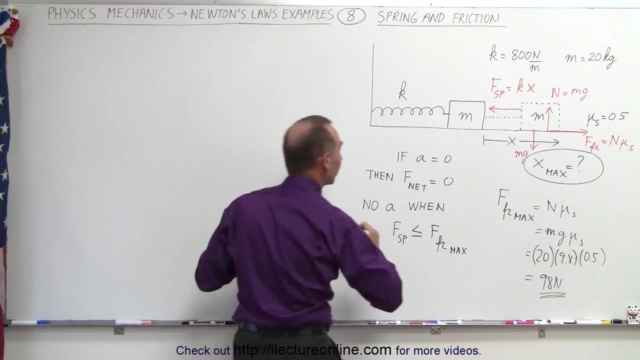 force equals maximum and what that equals the force caused by the spring, and so maybe i should put up the maximum friction force. as long as this is less than or equal to maximum friction force, it will not move, okay, so the force of the spring that's equal to kx has to be less than equal to the maximum. 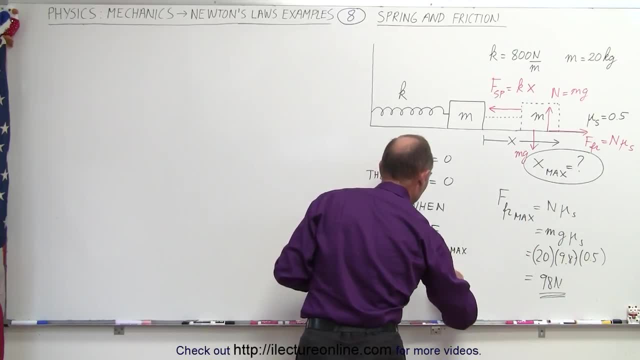 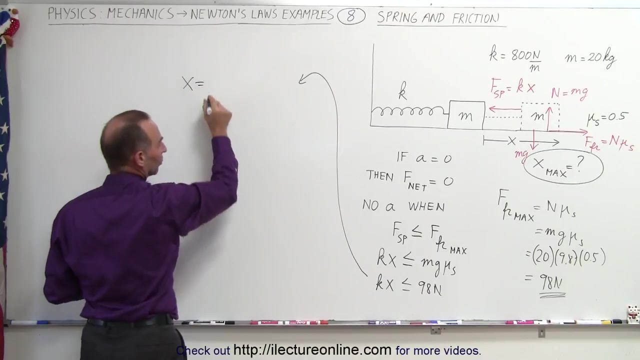 friction force, which in this case is going to be mg, mu, sub s or kx, has to be less than equal to 98 newtons, because that's the maximum the friction force can be. so when we come up here, we can then say that x is equal to the maximum friction force or less than or equal to 98 newton. 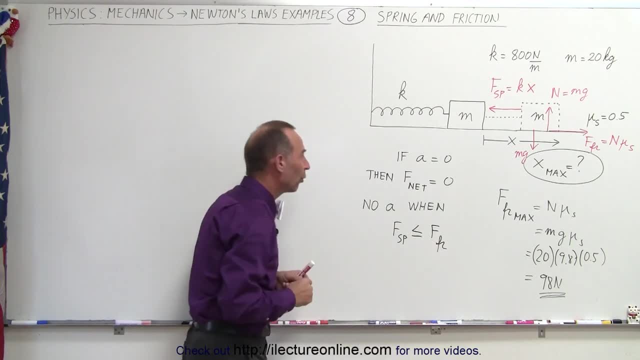 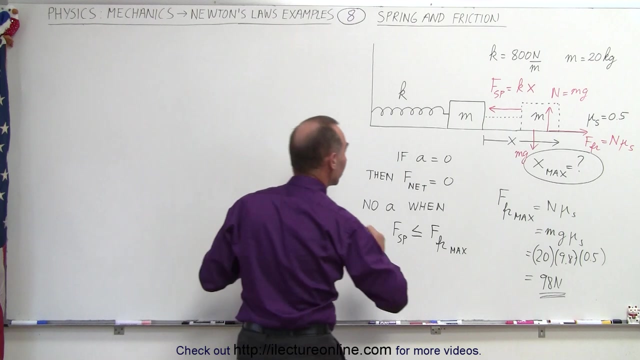 force equals maximum and what that equals the force caused by the spring. and so maybe i should put up the maximum friction force. as long as this is less than or equal to maximum friction force, it will not move, okay, so the force of the spring that's equal to kx has to be less than or equal to the maximum. 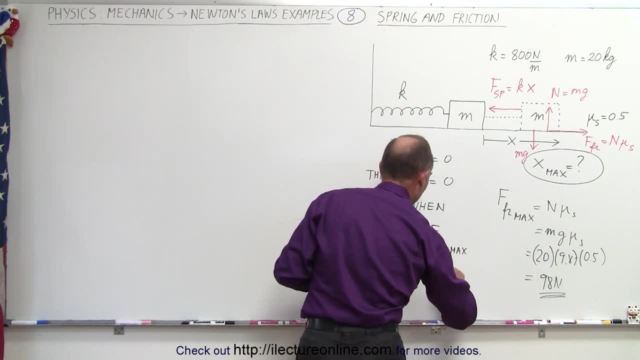 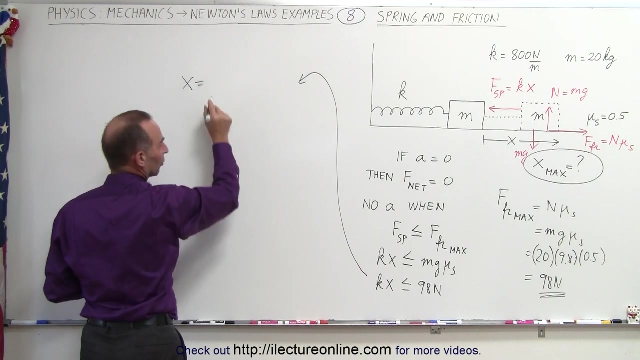 friction force, which in this case is going to be mg, mu, sub s or kx, has to be less than or equal to 98 newtons, because that's the maximum the friction force can be. so when we come up here, we can then say that x is equal to the maximum friction force or less than or equal to 98 newtons. 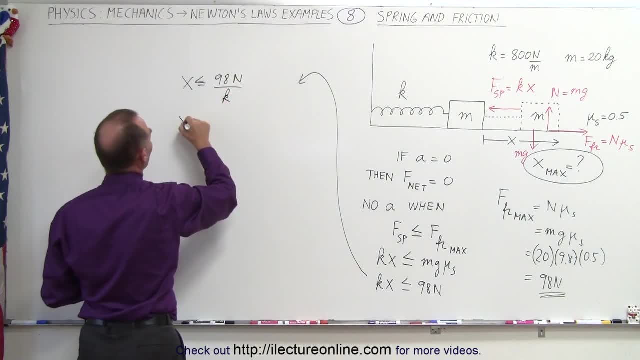 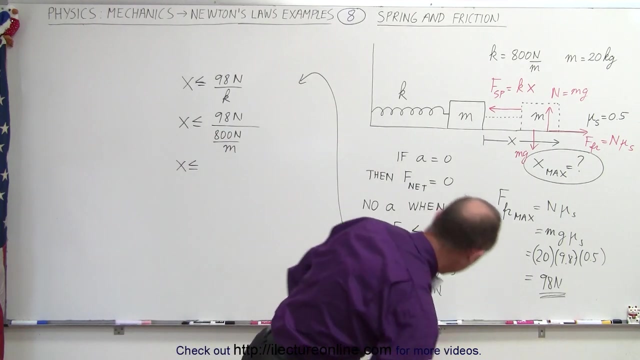 divided by K, and so X has to be less than or equal to 98 newtons divided by 800 newtons per meter, and of course X will be less than or equal to. that will then be in meters. so 98 divided by 800 equals. 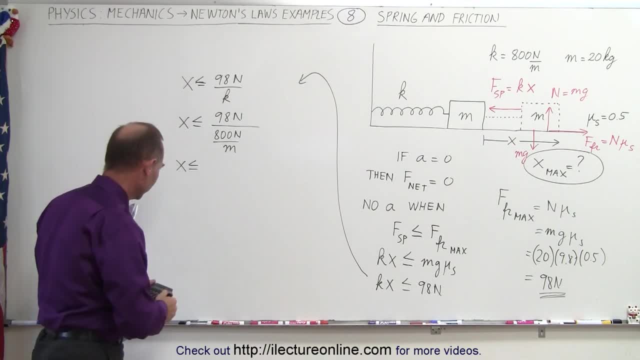 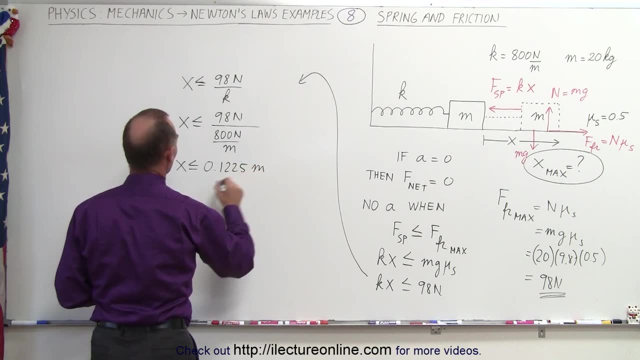 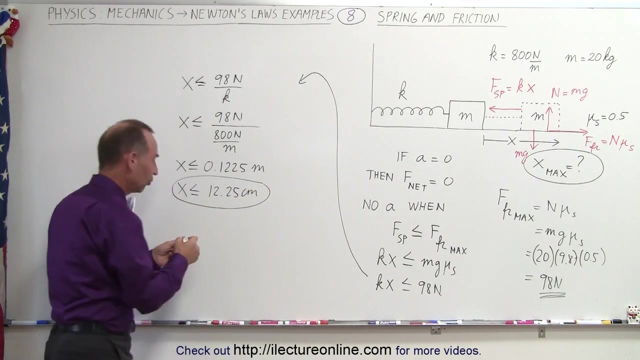 eight zero point one, two, two, five meters. so less than zero point one two, two, five meters. or X should be less than or equal to twelve point two, five centimeters. as long as the distance you pull the mass out it's less than twelve point two, five centimeters and you let go, the block will stay. 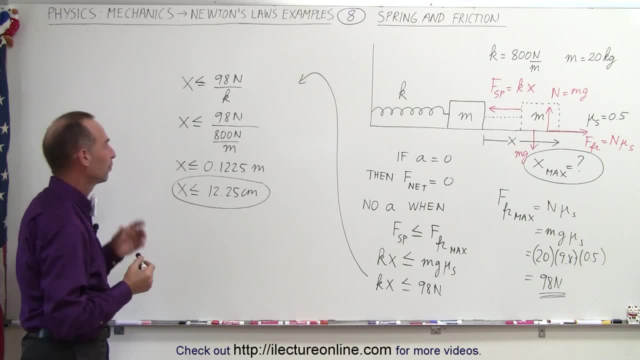 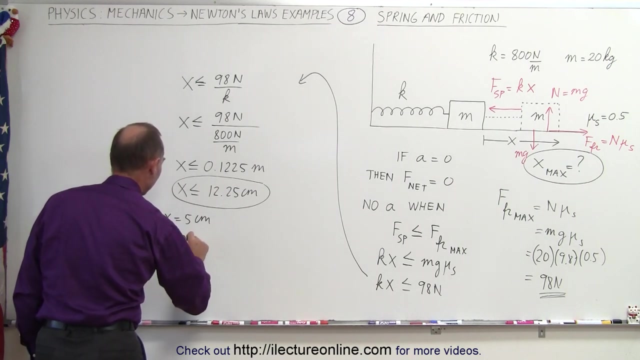 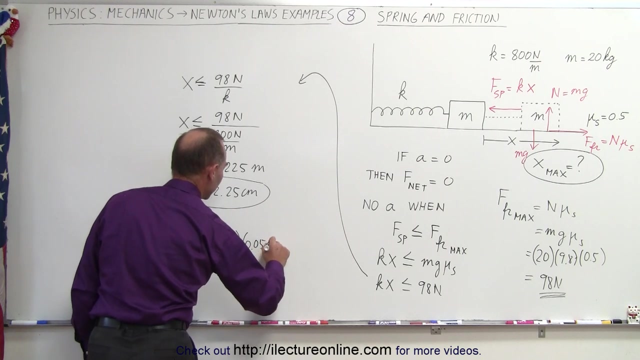 in place. so what does that mean? well, let's see here. let's say that if X equals five centimeters, what will the force of the spring be then? F of the spring will be equal to K times X, which is equal to 800 newtons per meter times 0.05 meters, which is equal to 40. 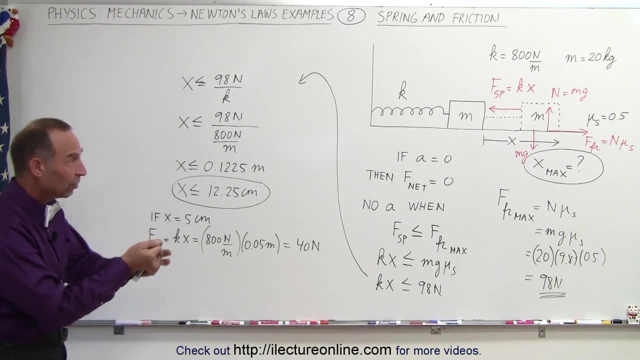 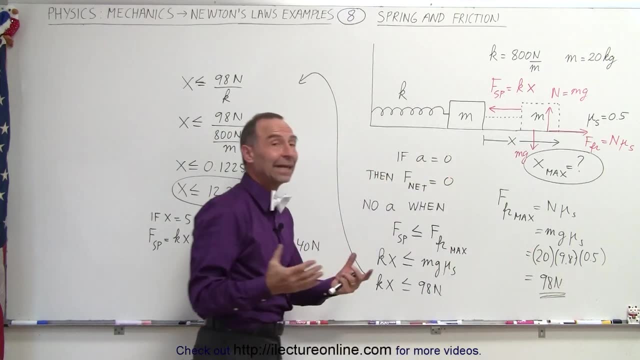 newtons. so when you pull the block out five centimeters, the force and spring will be 40 newtons. since the maximum force at the that the friction force can be is 98 newtons, it's less than the maximum. the block will not move. what will be? 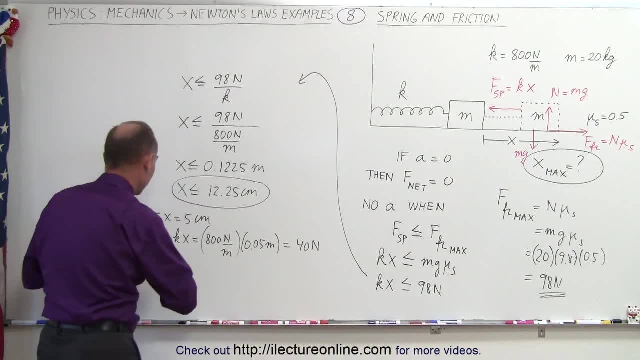 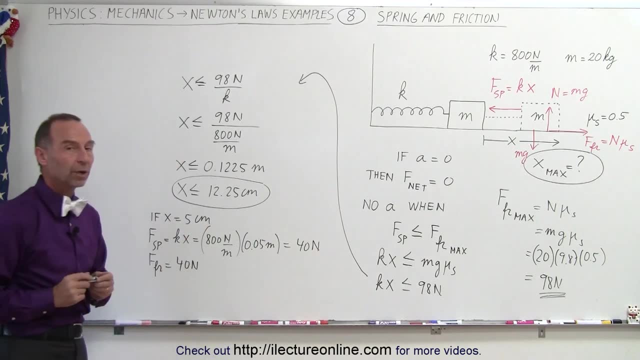 the friction force at that moment. well, it turns out that friction force at that moment, force friction will also be 40 newtons, because it will simply match the force of the spring. now what happens? that if X equals 10 centimeters, then the force due to this of the spring is equal to K times X, which 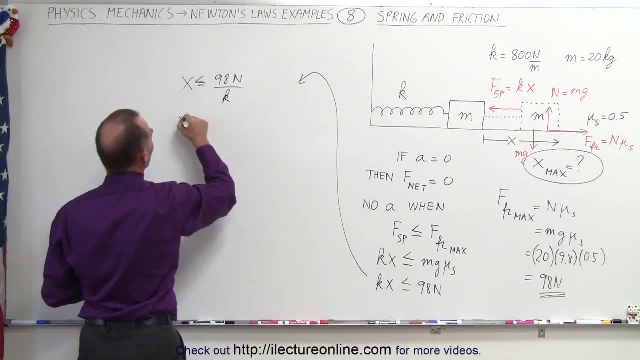 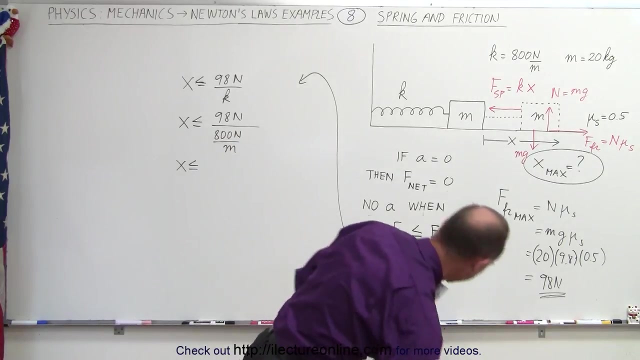 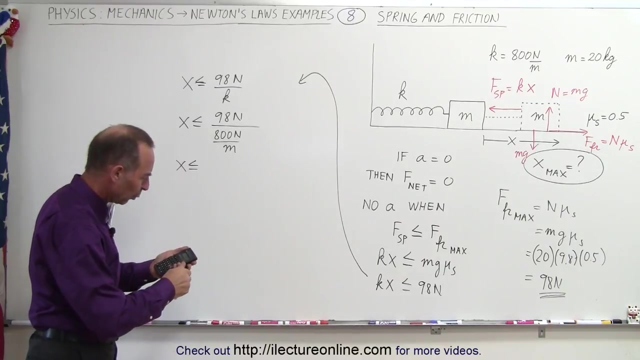 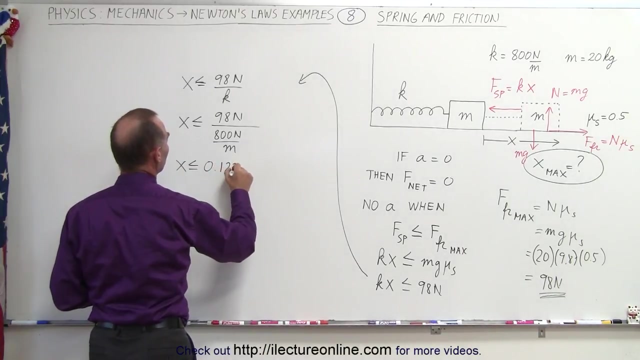 divided by K, and so X has to be less than or equal to 98 Newtons divided by 800 Newtons per meter, and of course X will be less than or equal to. that will then be in meters. so 98 divided by 800 equals eight, zero point one, two, two, five meters, so less than 0.12, two, five meters or X. 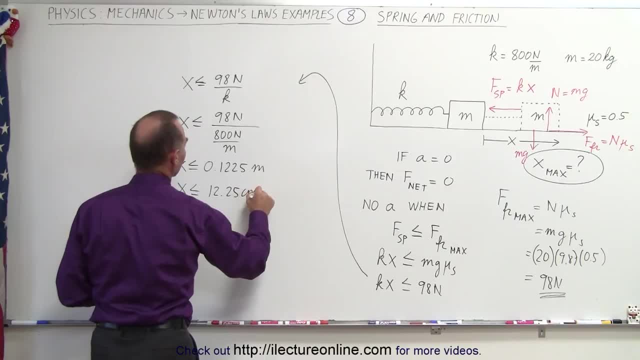 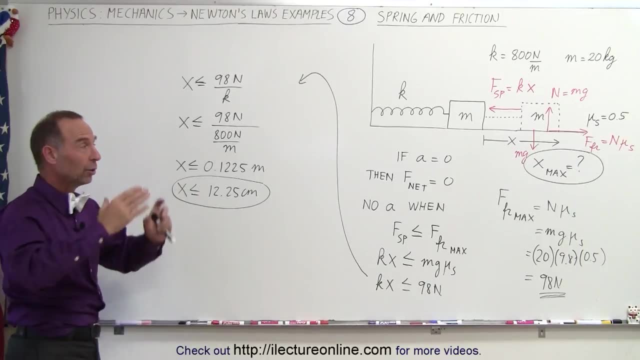 should be less than or equal to twelve point two, five centimeters. as long as the distance you pull the mass out, it's less than twelve point two, five centimeters and you let go, the block will stay in place. so what does that mean? well, let's see here. let's say that. 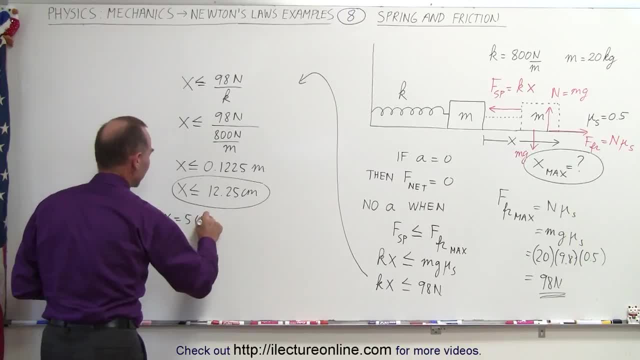 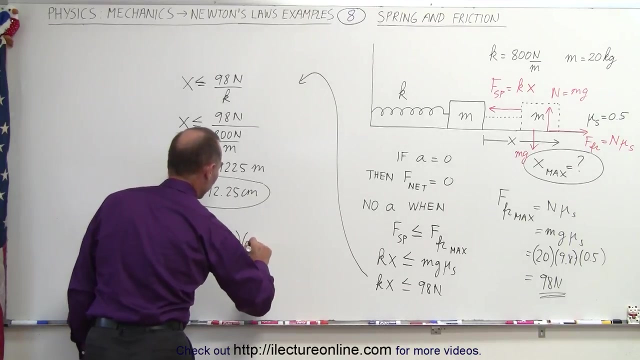 And if x equals 5 centimeters, what will the force of the spring be Then? f of the spring will be equal to k times x, which is equal to 800 newtons per meter times 0.05 meters, which is equal to 40 newtons. 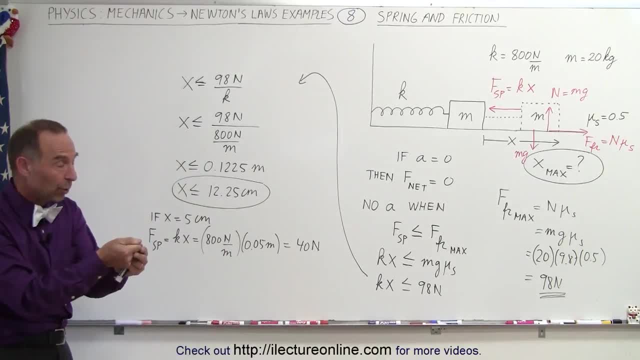 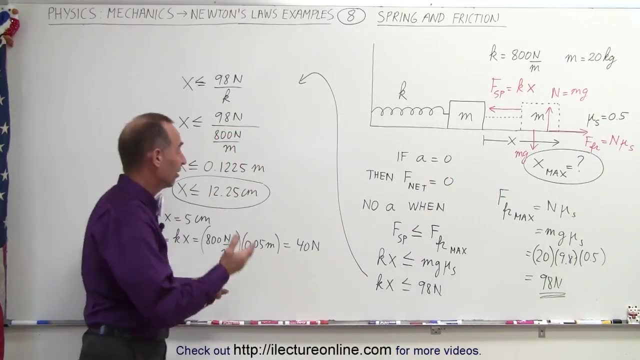 So when you pull the block out 5 centimeters, the force of the spring will be 40 newtons. Since the maximum force that the friction force can be is 98 newtons- it's less than the maximum- the block will not move. 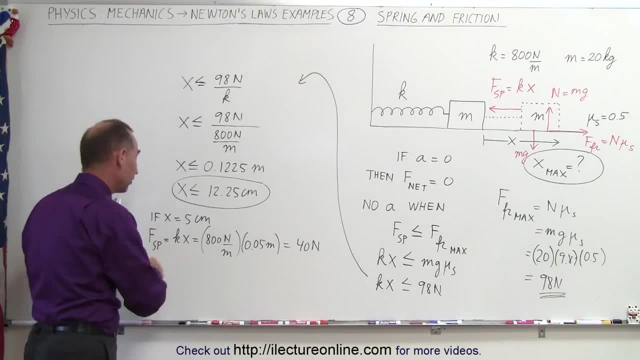 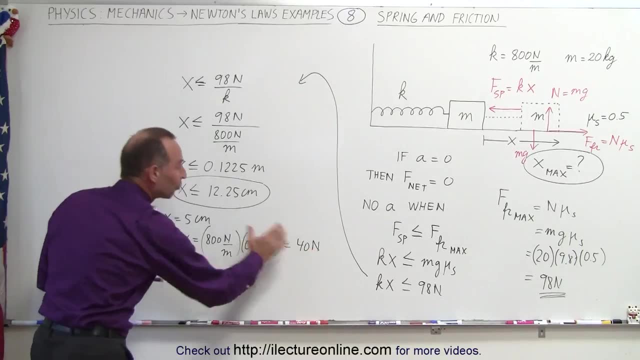 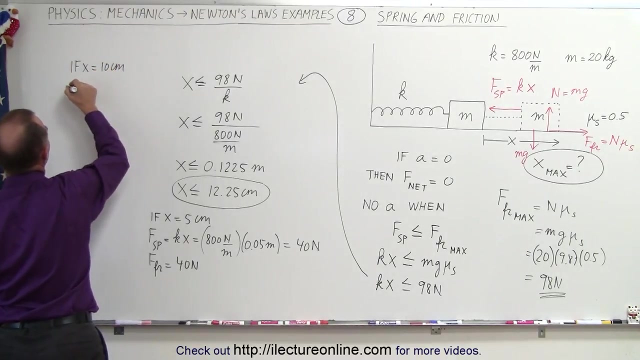 What will be the friction force at that moment? Well, it turns out that friction force at that moment, force friction will also be 40 newtons, because it will simply match the force of the spring. Now what happens? that if x equals 10 centimeters, then the force due to the spring is equal to k times x. 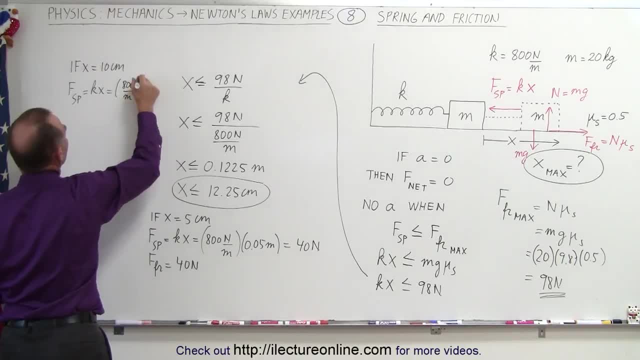 Which is equal to 800 newtons per meter times 0.1 meters. because 10 centimeters is 0.1 meters, That will be equal to 80 newtons. Notice that it's still less than the maximum the friction force can be. 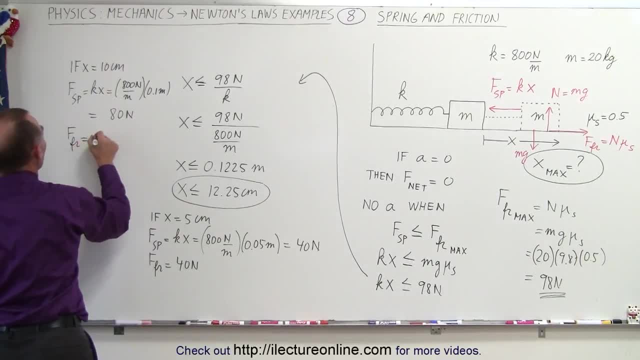 And then you can say that the force, friction, will also be 80 newtons, because, again, the friction force is simply a reaction force, Newton's third law: If the force applied by the spring is 80 newtons, the spring, the friction force, will pull back with a force of 80 newtons.